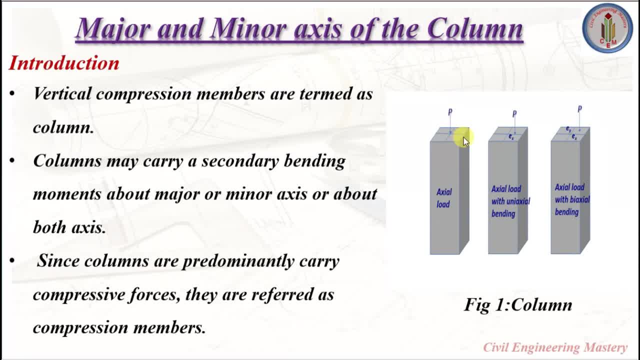 is symmetrical, so there will not be any moments. Though the columns are predominant with axial force, the columns may also carry a secondary bending moment about major axis or minor axis, or about both axis as well. So if the column is carrying the moment about either one of the axes, 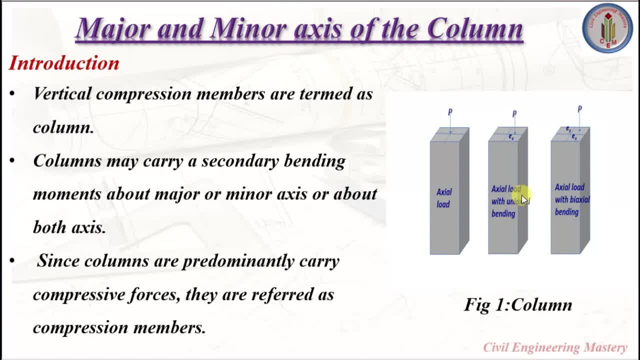 axis or minor axis, then we call it as a uniaxial bending. if the column is carrying the moment about both the axis, then we call it as a biaxial bend. so in order to design the column with moments, we need to know which is major axis moment and which is minor axis moment of the column. so this is the 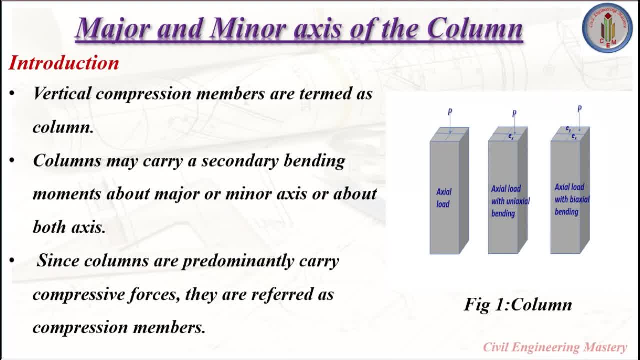 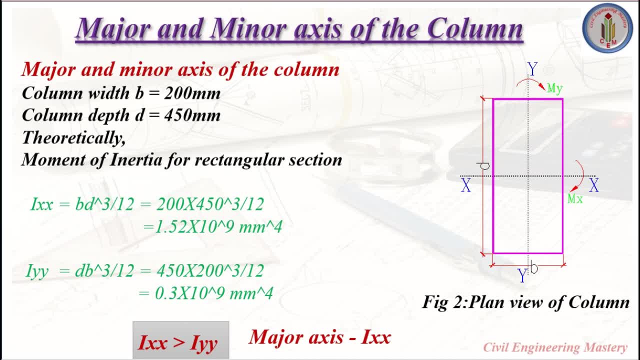 reason we are discussing how to find out the major and minor axis of the column. now let us discuss how to find out the major and minor axis of the column. the column dimensions are given here. column width is 200 mm. column depth is 450 mm. theoretically, the major and minor axis of the rectangular 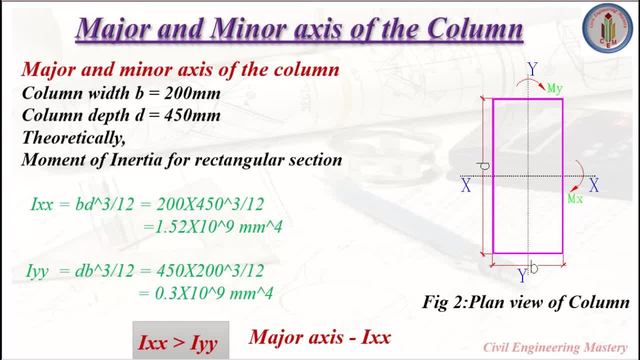 section can be found out by using moment of inertia. so the formulas are given here: the moment of inertia for x axis, that is, ixx, is equal to bdq by 12 for this rectangular section, and iyy is equal to dbq by 12. so if we apply these, 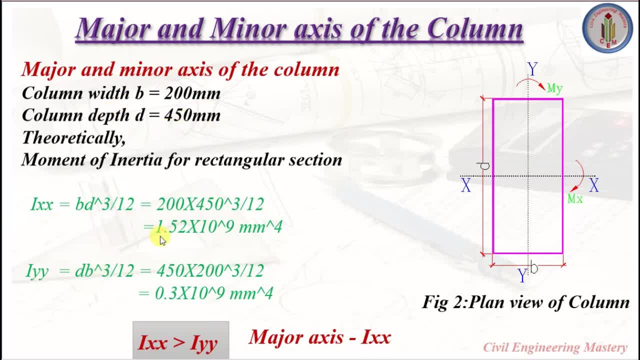 bdq by 12 for this rectangular section and iyy is equal to bdq by 12. so if we apply these bdq by 12 value in this formula, we get the Ixx value as 1.52 multiplied by 10 to the power 9 mm. power 4. 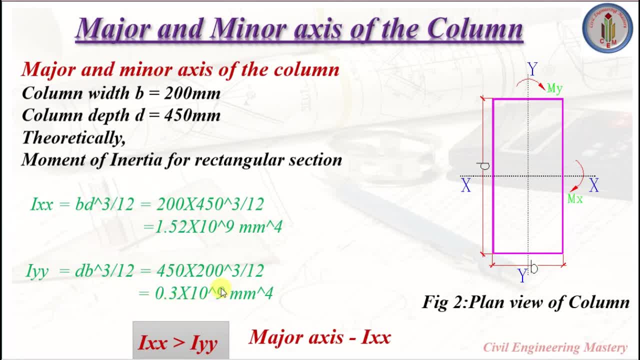 and Iyy value is 0.3 multiplied by 10 to the power: 9 mm, power 4.. So if we compare these two values, Ixx is the greater value and Iyy is the lesser value. So we can come to know that Ixx is the. 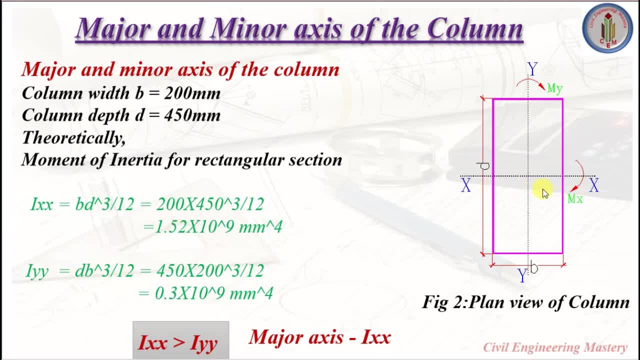 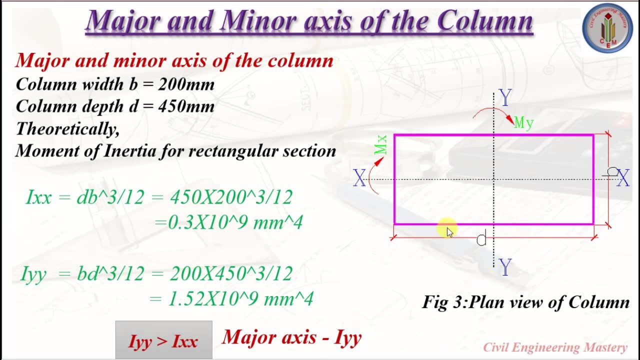 major axis. From this figure we can say that the axis which is perpendicular to the depth of the section is major axis and the axis which is parallel to the depth of the section is minor axis. Now see, here, the orientation of the section is different here. So if we find out the major and 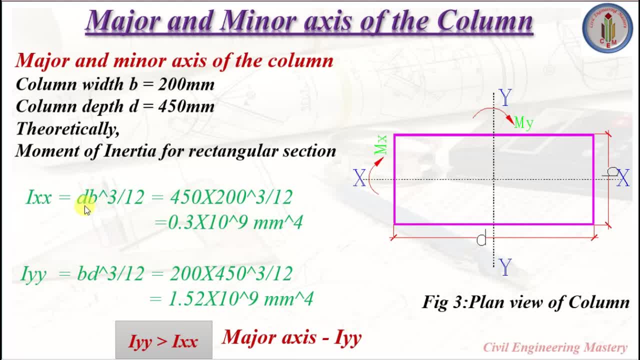 minor axis of this section by using moment of inertia. Ixx is equal to 0.3 multiplied by 10, to to dB cube by 12, and Iyy is equal to Bd cube by 12.. So the values are different here. Ixx has the 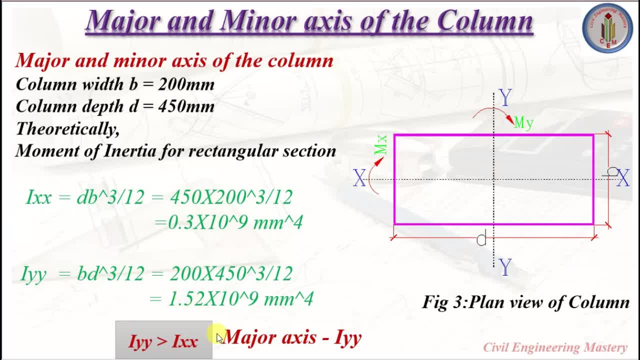 lower value and Iyy has the higher value. So here the major axis is Iyy. From this figure we can say that the axis- see this is the axis which is perpendicular to the depth of the column. Y axis is the major axis, So which is perpendicular to the depth of the column, and x axis is the minor. 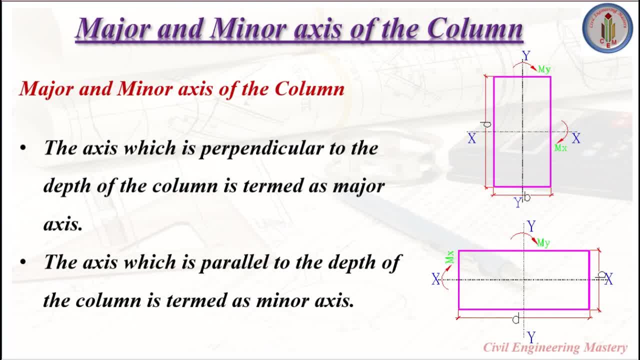 axis which is parallel to the depth of the column. Practically, we can say that the axis which is perpendicular to the depth of the column is termed as major axis and the axis which is parallel to the depth of the column is termed as minor axis. Once again, let's recall with this section which 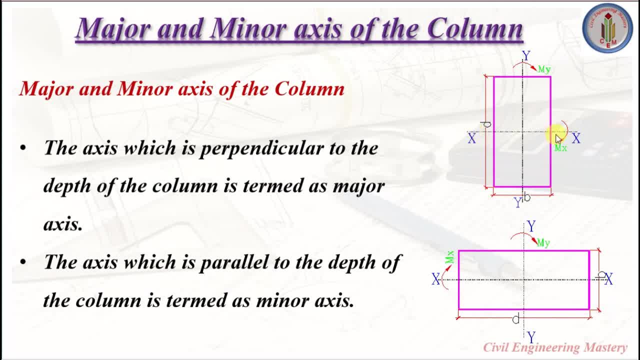 is major axis and which is minor axis. So here for this section, you can see that the axis which is perpendicular to the depth of the column is termed as minor axis. This is the axis which is perpendicular to the depth of the column, So it is called as major axis. 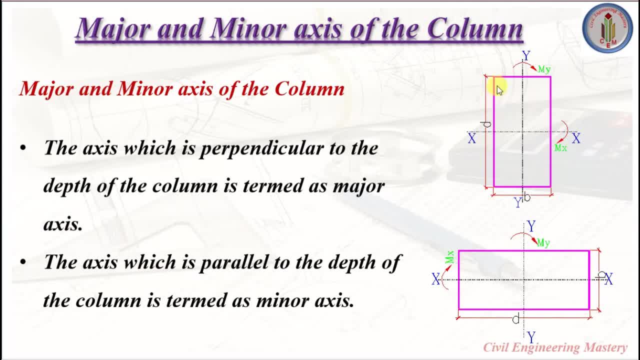 and y axis is the axis which is parallel to the depth of the column, So it is called as minor axis, and for this section it is different. Here the axis- the y axis- is the perpendicular to the depth of the column, So it is called as major axis, and x axis is the parallel to the depth of the. 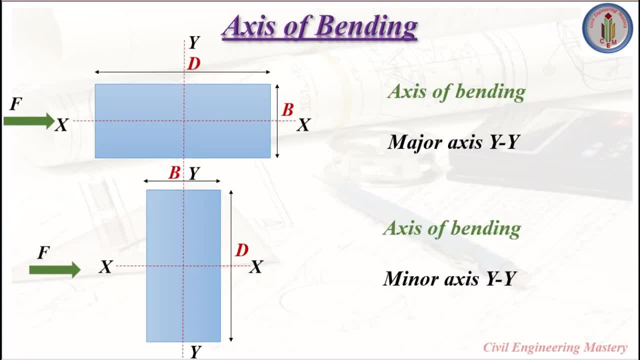 column, So it is called as minor axis. Next let us discuss about axis of bending. Consider the force F which is applied on this direction, on the column, how the column bends. the column bends in this way, So here the axis of bending is major axis, that is y, y. 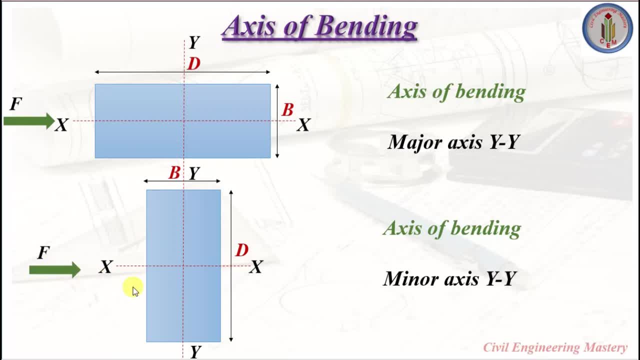 Next, consider the force which is applied on this column in this direction. So how the column bends in this way. So here the axis of bending is minor axis, which is y? y Hope all of you have clearly understand about how to find out the major and minor axis of. 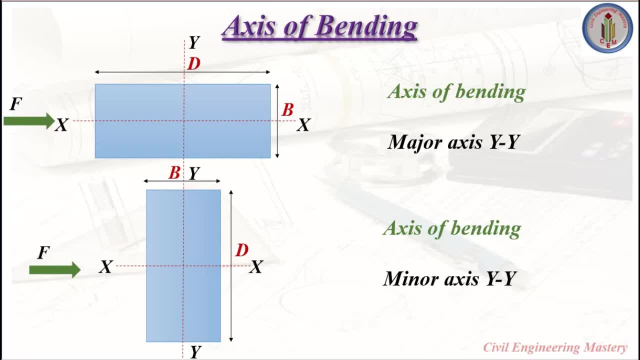 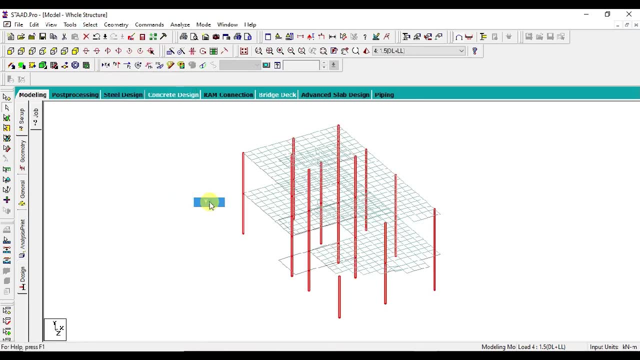 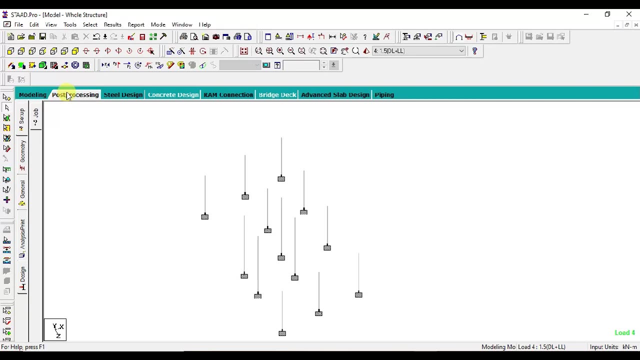 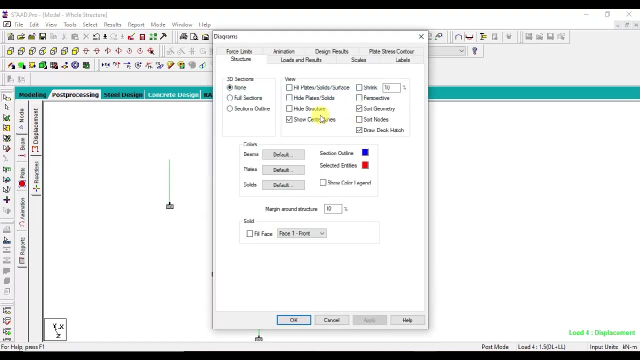 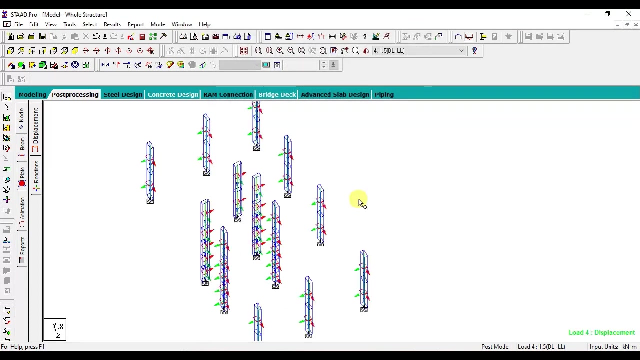 the column. Now let us discuss how to get the moment values from StarPro software. Go to select beams parallel to y. So we are selecting only columns. for better understanding, Go to post processing mode And here right click on the column, Right click structural diagrams, Section outline And under label beam orientation. 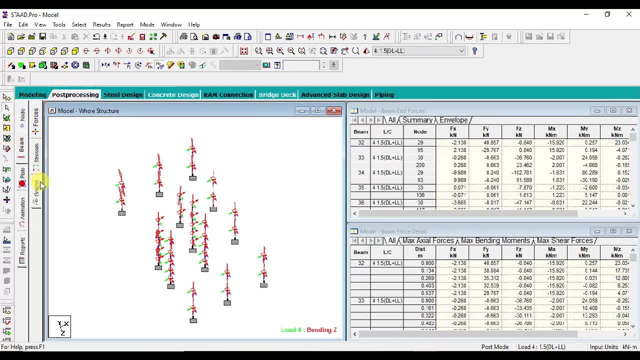 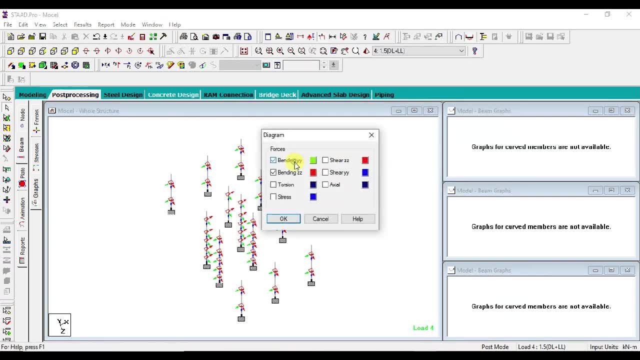 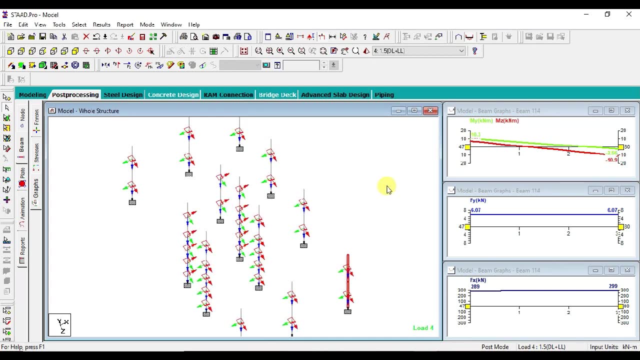 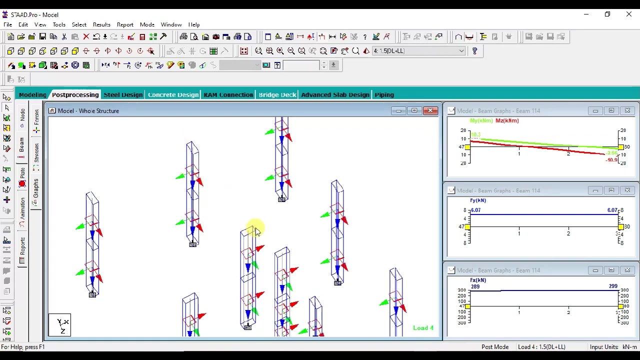 Ok, And here go to beams graphs. Right click diagrams bending y, y so that we get both values: m y and m z. So here we need the section outline again. Ok, Now see, the columns are oriented in both direction: In this direction as well as in this direction. 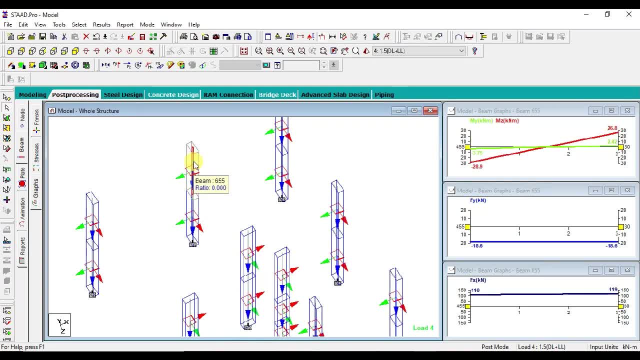 So if you take this column select, you can see the moment values m y and m z. So here which is the major axis, this green color that is, m y is the major axis and m z is the minor axis. So the moment values are given here. Major axis value is 3.75 and minor axis value 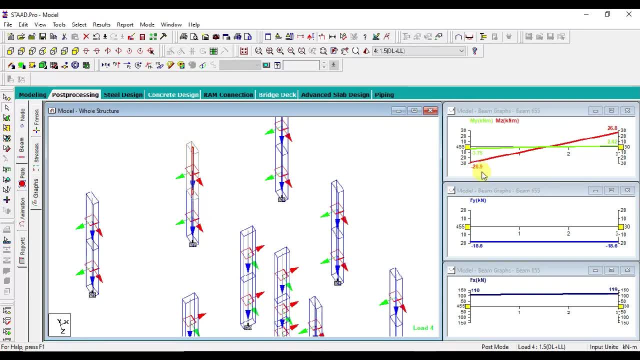 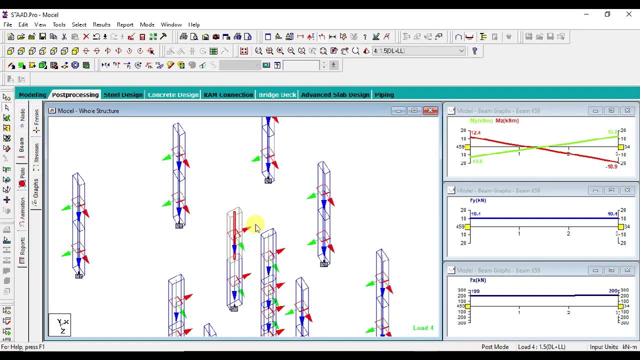 is 28.9 kNm. So if you take this column, Here the orientation is different And here the major axis is again m y and minor axis is m z. So m y value is the maximum is point 2 and M is at value. maximum is 18.9. so this is how we have to get the 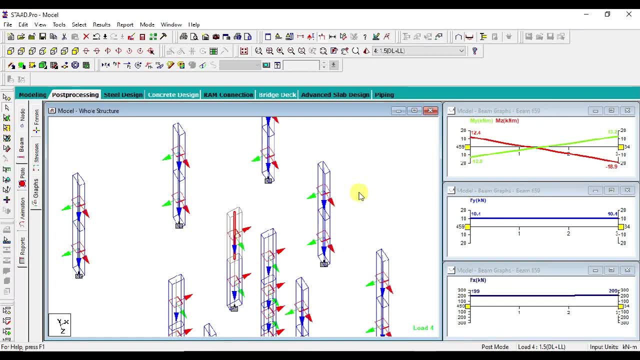 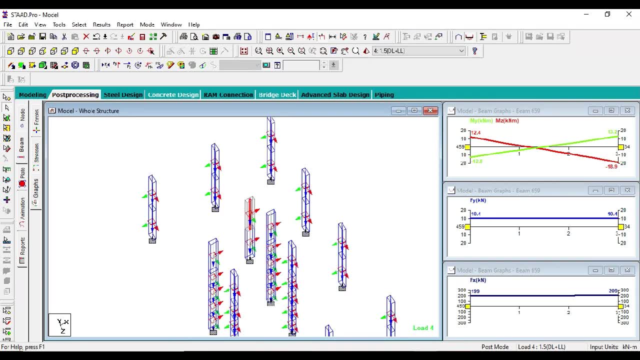 major and minor axis moment values from this software in order to design the column with moments. friends, hope all of you like this video. thank you for watching.